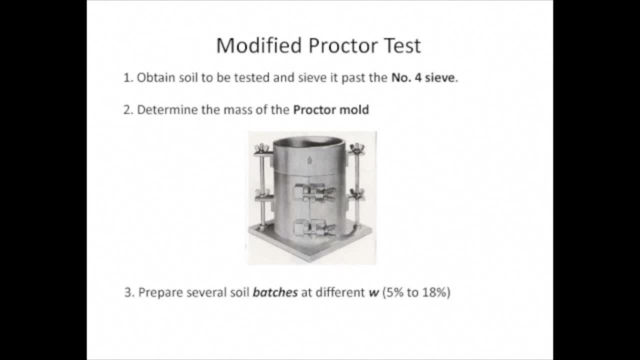 predecessor, the standard Proctor test. To perform the modified Proctor test, we do the following: We first obtain approximately 40 pounds of soil that passes the number 4 sieve, That is, all. the particles in the soil must be smaller than 4.76 millimeters. We then determine the mass of the Proctor steel. 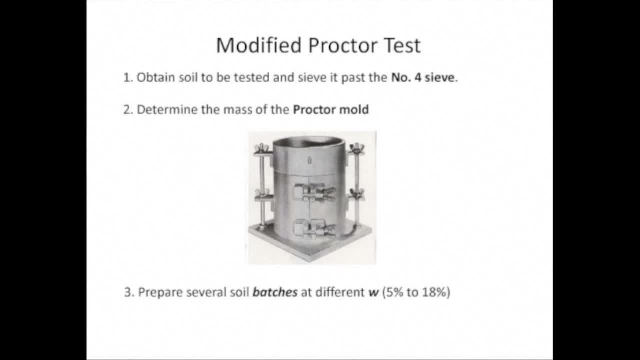 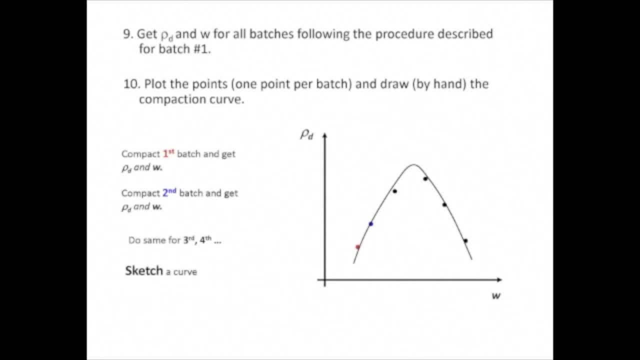 We then divide the soil into at least six separate batches and we add water or remove water by drying. We then create the compaction curve by plotting our points and drawing a best fit curve by hand. We then create the compaction curve by plotting our points and drawing a best fit curve by hand. 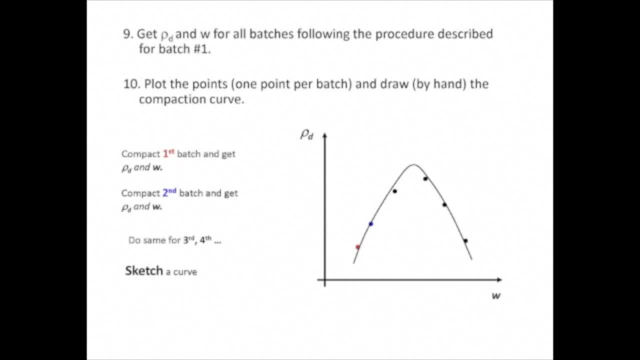 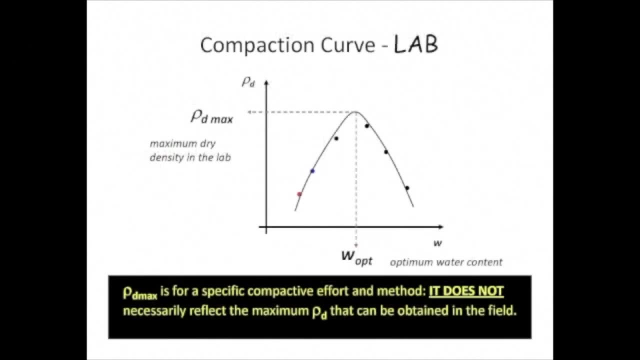 It is important that you do not simply join the points with lines. The Compaction Curve. The Compaction Curve is unique for a given soil type, used method of compaction and applied compactive effort. Notice that the curve has a peak, Therefore there is a compaction water content. 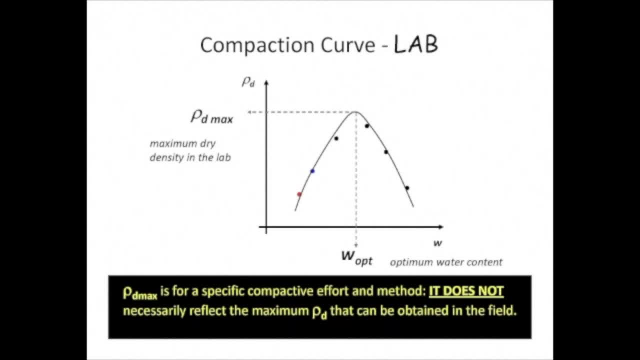 Therefore there is a compaction water content that optimizes the compaction process. That is to say, if the soil is compacted at the optimal water content, then the highest dry mass density achievable in the lab is obtained. This dry mass density is called the maximum dry density, rho d max. 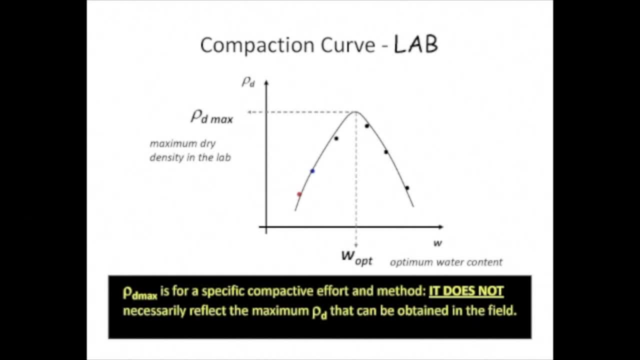 Rho d max is unique to a specific compactive effort and method. It does not necessarily reflect the maximum dry mass density that can be obtained in the field. This is because a different compactive effort and different means are used to compact the soil in the field. 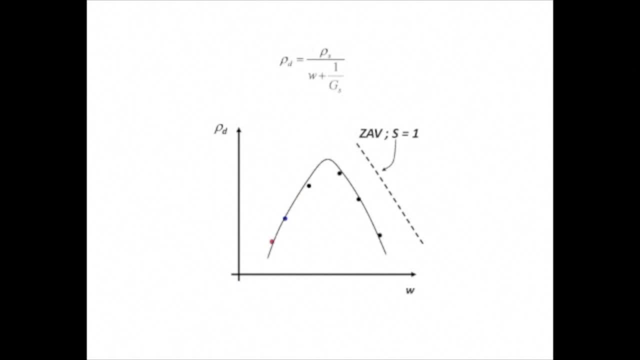 It is important to note that a soil compacted at the optimum water content is not fully saturated. That is, s is not equal to 1.. To visualize the level of saturation with which a soil is compacted in the lab, we plug in the d max. 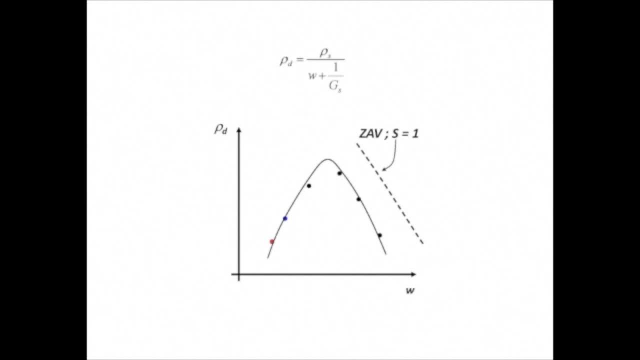 We put the so-called zero-ervoids curve, the ZAV, next to the compaction curve. We do so by using the following equation: The dry mass density is equal to the mass density of solids divided by the water content plus 1 over the specific gravity of solids. 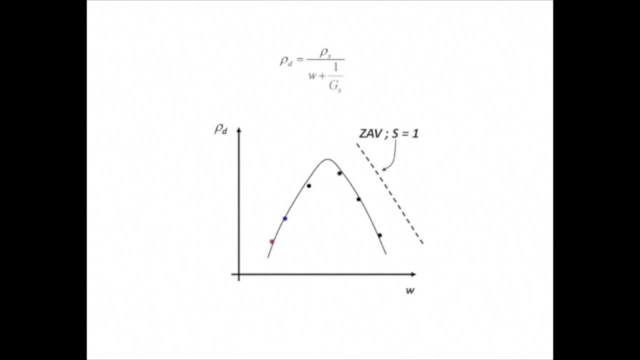 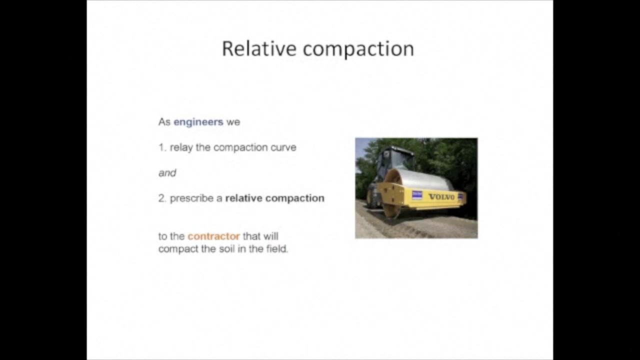 In this equation, the water content is a variable that is used to create the zero-ervoids curve. The ZAV must lie to the right of the compaction curve. as shown, As engineers, our primary job with respect to compaction is to give the contractor the information he or she requires to appropriately compact the soil in the field. 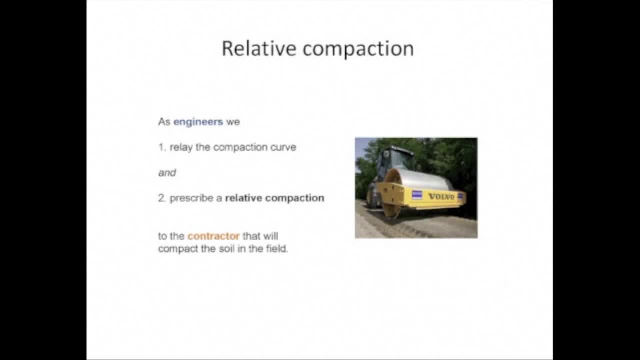 In general, the engineer relays the compaction curve to the contractor and suggests a range of water contents with which the contractor will be able to compact the soil efficiently in the field. In addition, the engineer prescribes a relative compaction for the project. 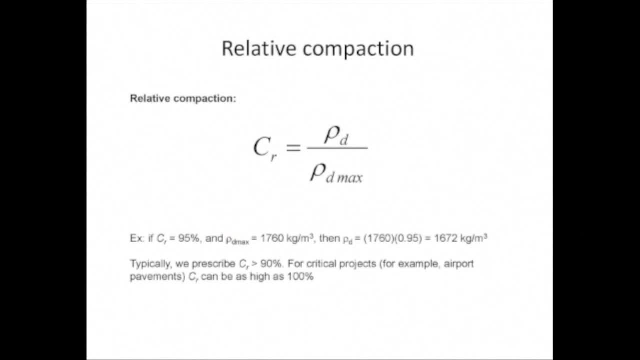 The relative compaction is the ratio of the dry mass density to be achieved in the field by the contractor to the dry mass density achieved in the lab. For example, let's say that a project calls for a relative compaction of 95%. The soil to be compacted in the field was tested in the lab. 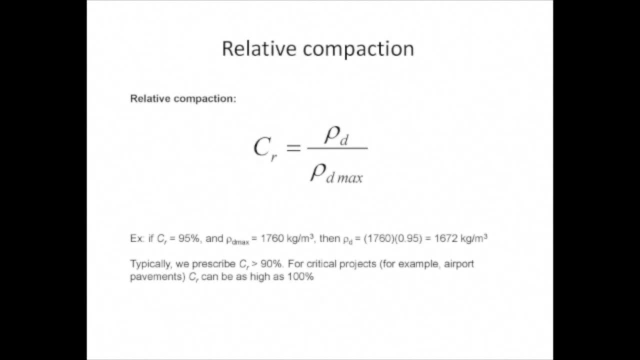 and the maximum dry density obtained using modified proctor was 1760 kg per meter cubed. This means that the soil must be compacted in the field to a dry mass density of at least 1672 kg per meter cubed. In general, relative compaction figures are above 90%. 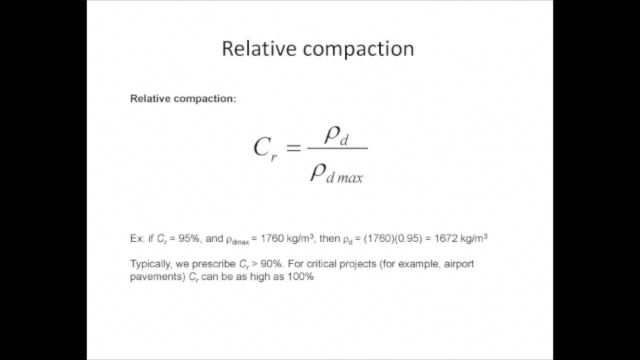 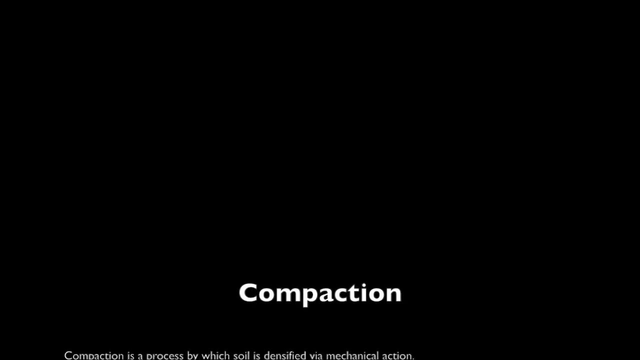 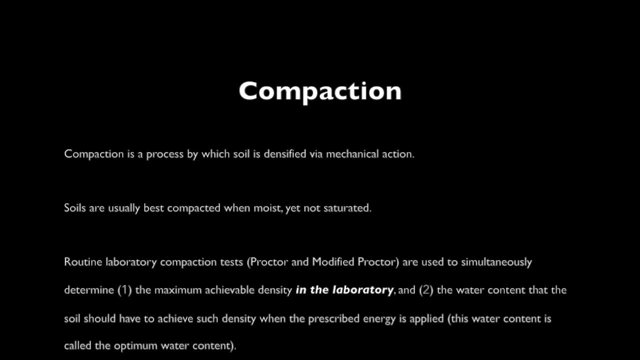 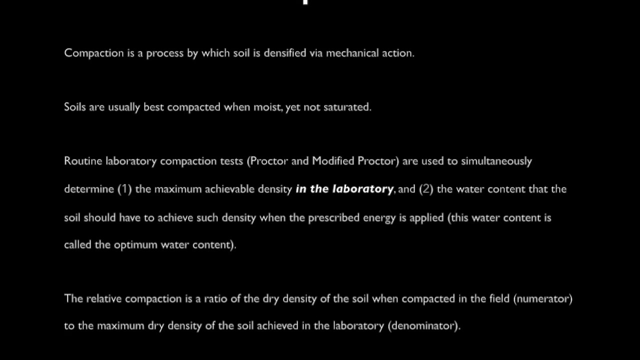 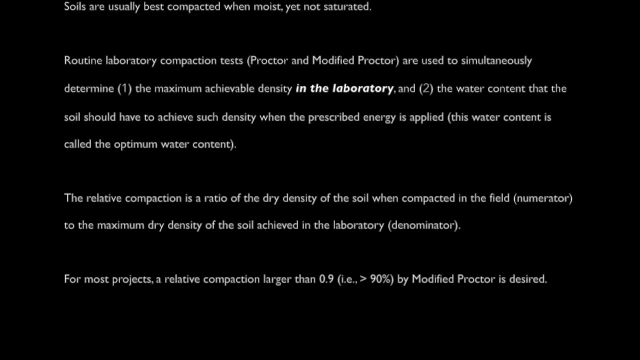 The prescribed relative compaction is dependent on the project in question. The relative compaction figure is composed of the following results: The反波 hour of the unit is 1.33 µm. The ratio of the value of the final range is 1.13.. 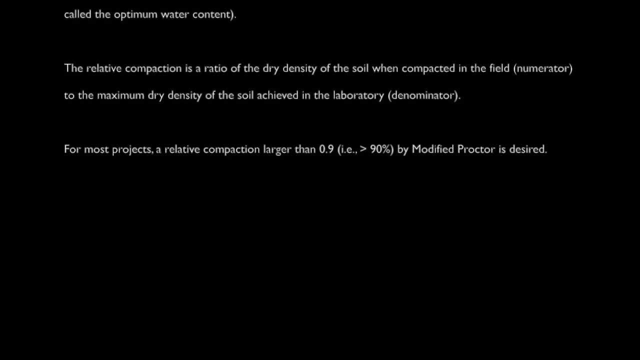 The ratio of the value of the unit is 1.28.. Thank you.